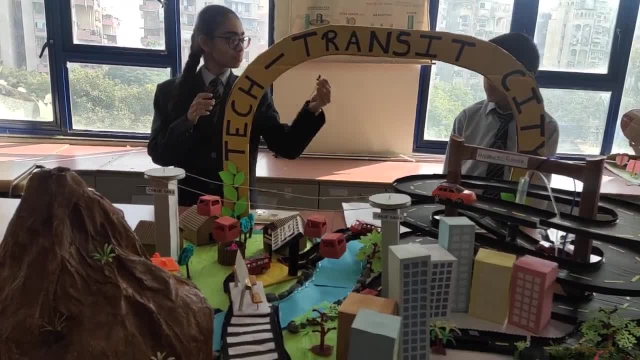 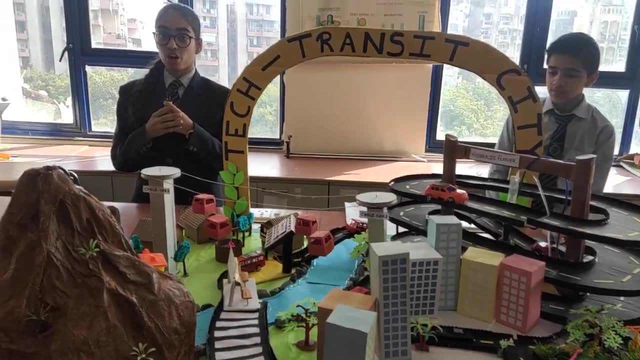 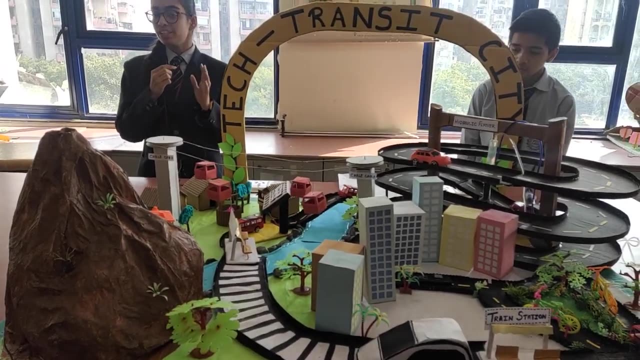 Greetings of the day. I'm Himali Tabas of class 8th and I'm Saksham Rati of class 7th P. Today we have prepared a model for science exhibition on the topic transport and innovation. We have prepared the city named as Tech Transit City. It's just like its name suggests: Tech means. 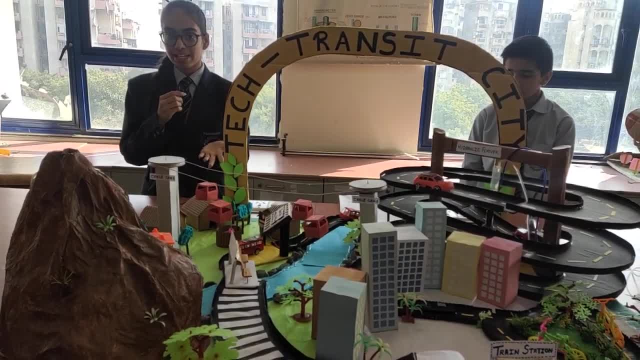 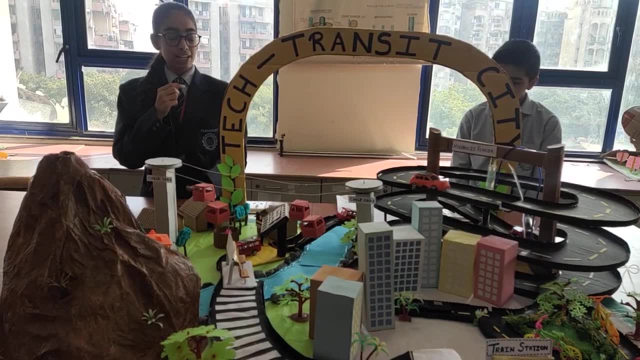 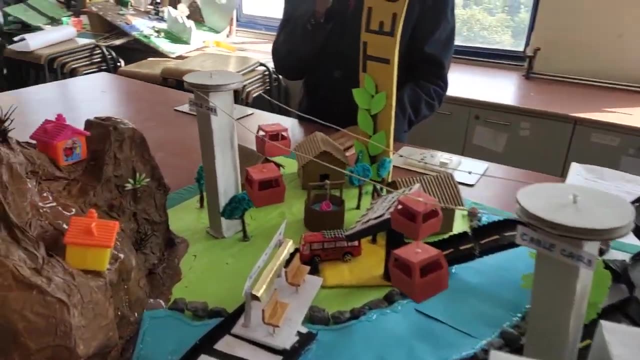 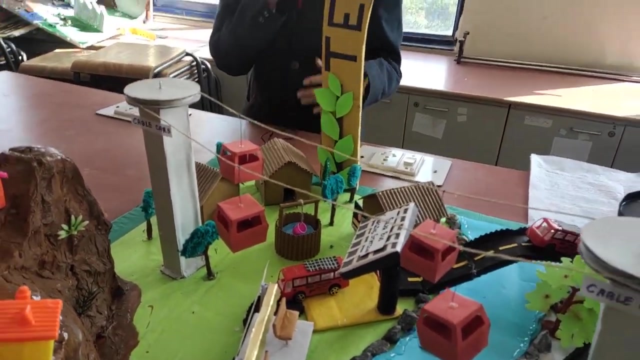 technology. transit means transportation and city means a large and important town. This city shows the development of transportation system and it also shows the connection of city with remote areas like villages and mountains. People can freely travel anywhere: from the city to the remote areas and from the remote areas to the city. This would benefit both of them. People living in remote areas. 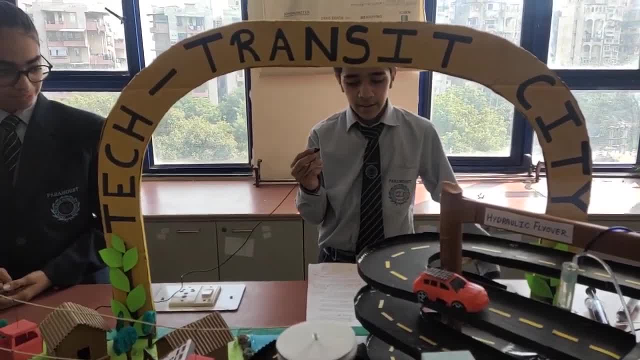 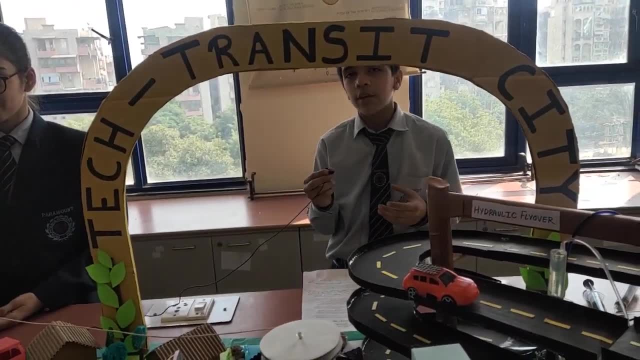 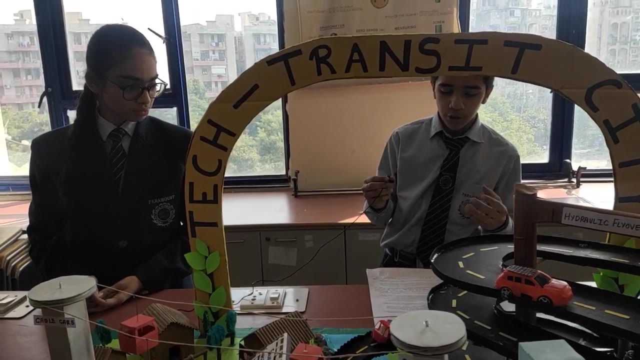 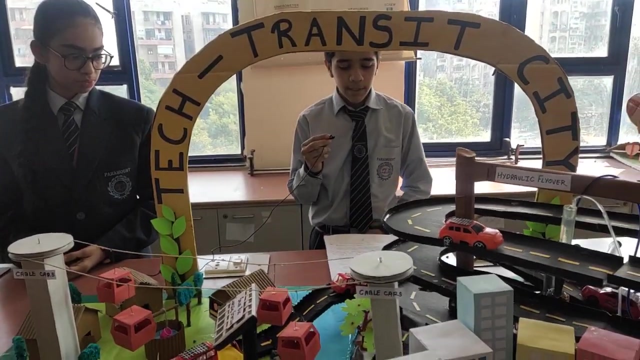 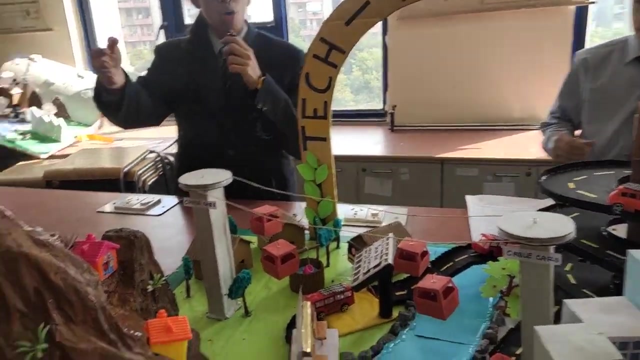 would get access to better resources and job opportunities, and whereas the people living in the cities could get the more manpower to share their workload. Along with these, it will also result in better education opportunities, healthcare will as the customer service. These new ideas are environment friendly as they do not cause any pollution and and saves the energy Over here. 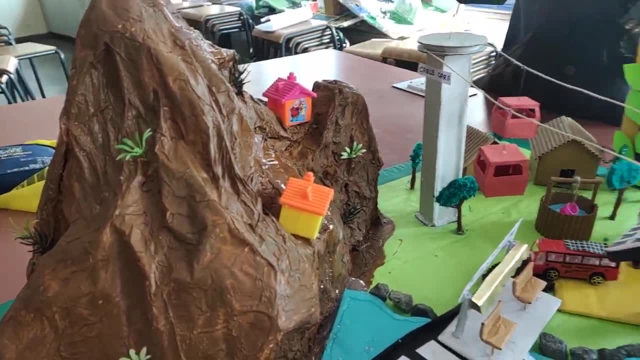 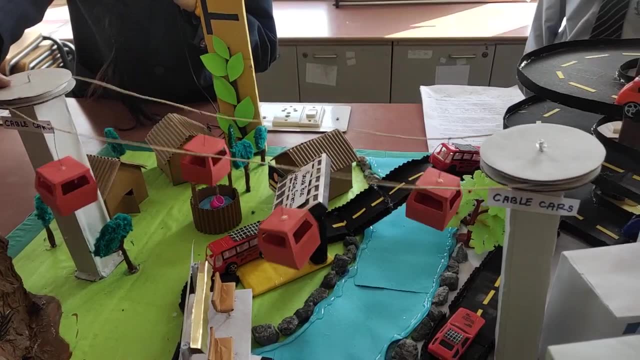 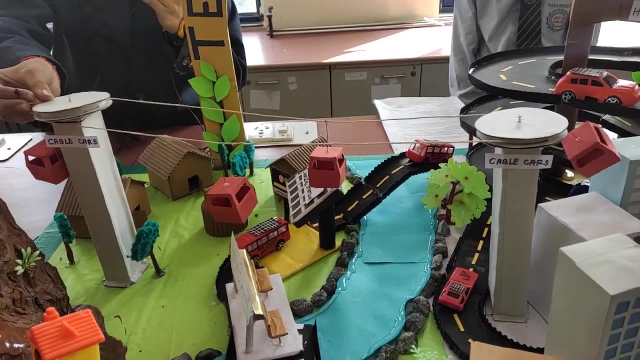 we have mountains. People living in the mountains can travel to the city using the cable cars. When the disk at one end is rotated, it creates rotatory motion. This rotatory motion is passed to the to the other disk through the thread tied around it, and this is how the cable car moves and that 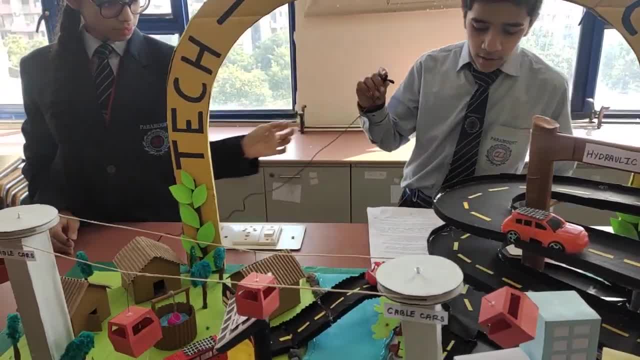 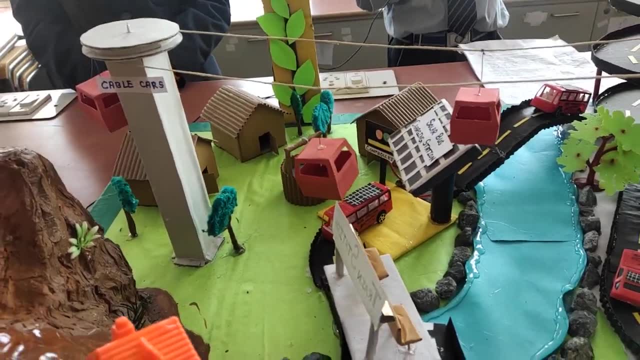 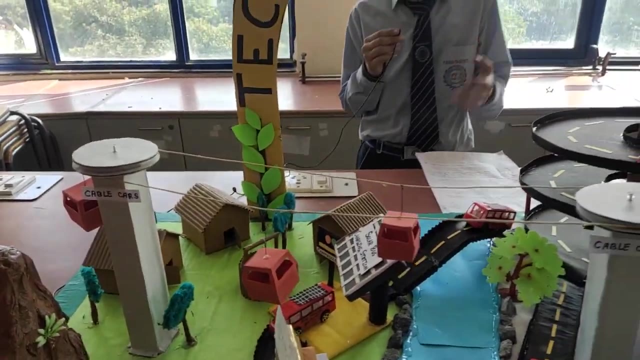 and carries people to the city. Here we have the villages and villages in the villages. uh, they are often power cuts and the electricity isn't always available. uh, available to the run. these batteries, electric buses we have provided, so we have a dual functioning bus. 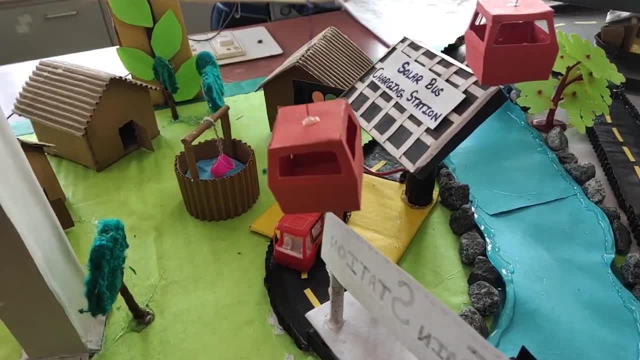 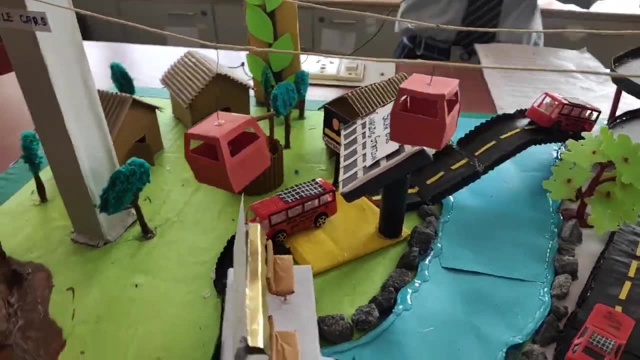 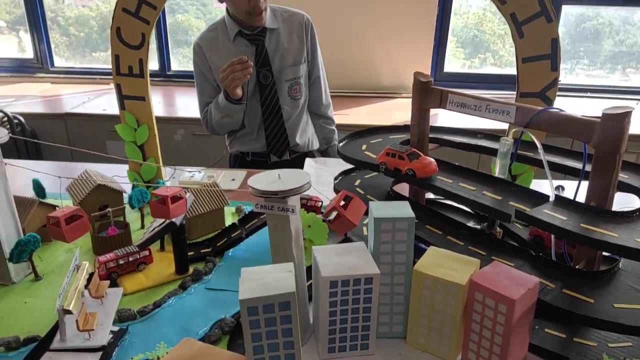 It its work on an electricity bus. in the absence of the electricity, it works with its solar panels. Solar panels comprises of many small photocells, photocells. photovoltaic cells means that they can convert sunlight into electricity, and these cells are made of semi-conductive. 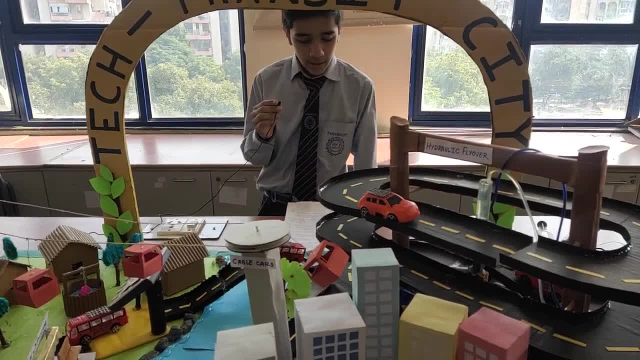 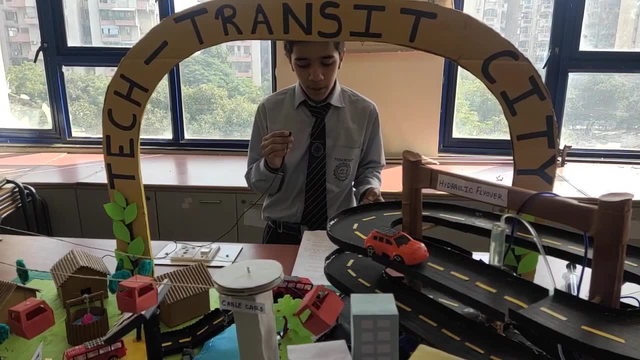 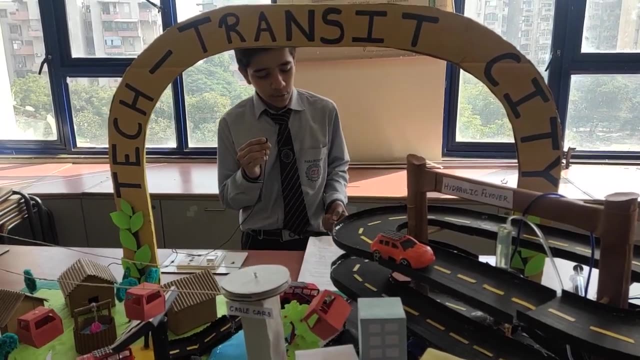 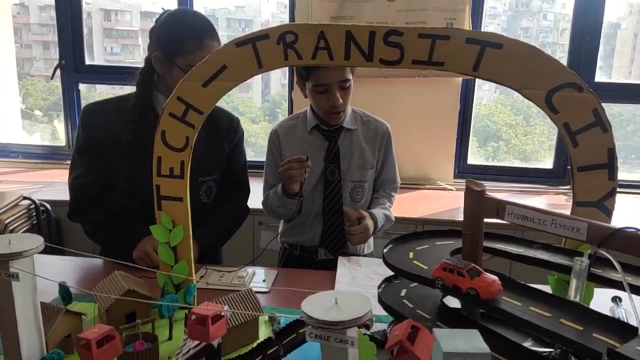 material, Most of silicon, are material that can conduct electricity. Photovoltaic cells bypass the original principle of the solar thermal uh material energy of the converting solar energy directly to usable electricity inside the thermal conservation. Therefore we can easily store the convert converted electricity in the batteries and use them in a power of engine or vehicle. 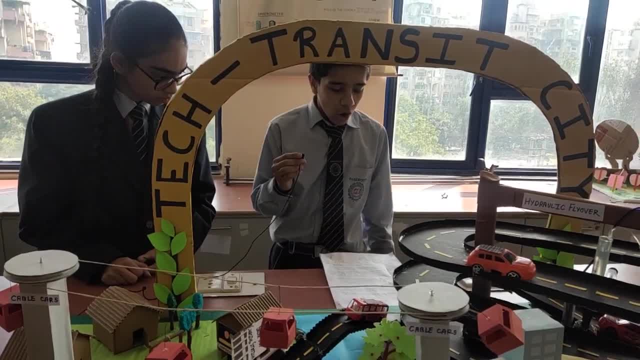 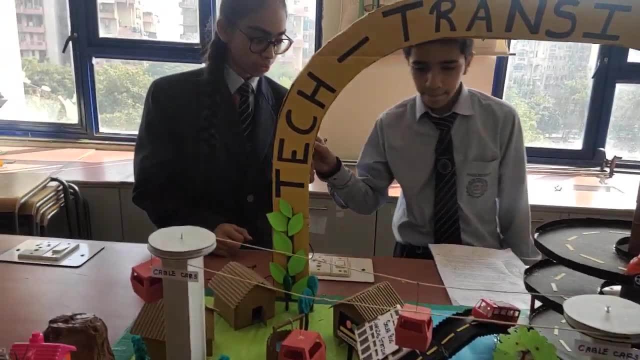 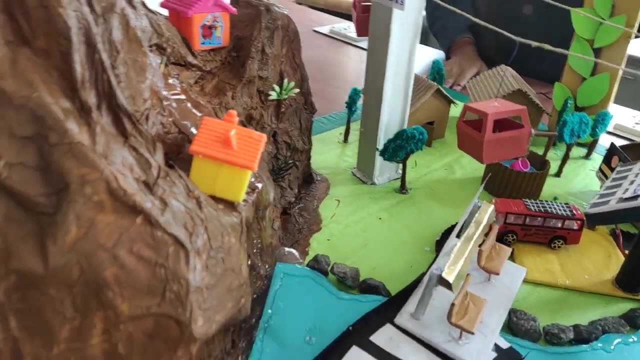 to out circulation of the vehicle just like a normal cars and buses. on solar buses charging stations, buses get time to recharge by the sunlight. People living in the village can use these solar buses to reach the train station. On reaching the train station they can get easily access to the electric train. electric train works. 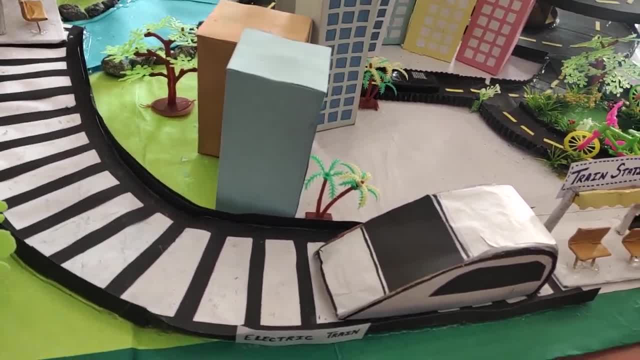 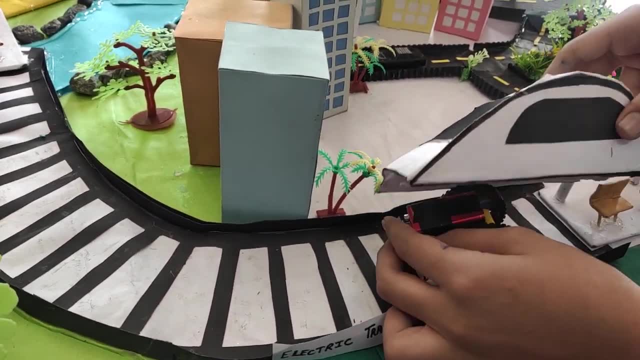 when electric train works, through the metal rods on the electric train bed, electric train pots, electricerie, weights, tires on the electric train. because it works, um you can easily the electric railway on the electric railway path. electric current flows through the railway path and it goes to the metal wheel. metal wheel is corrected, connected to the motor and when the 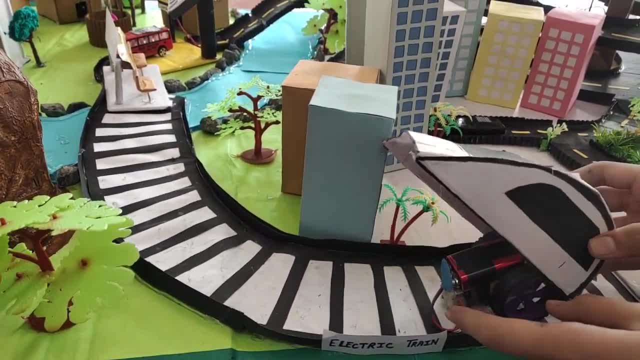 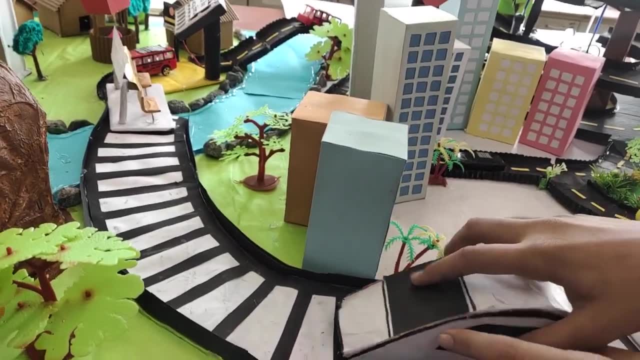 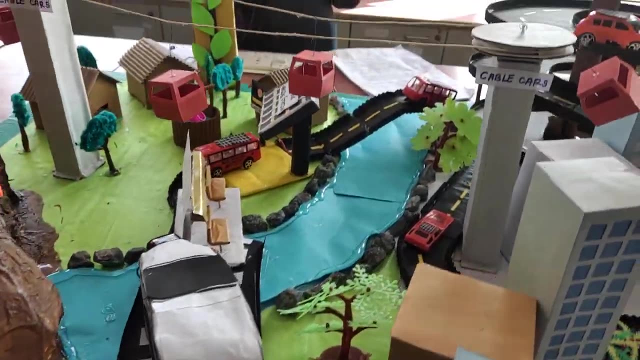 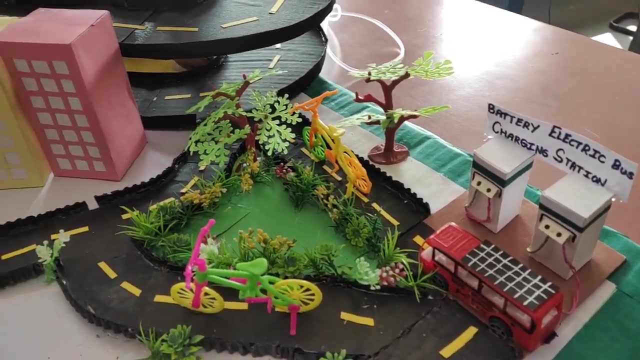 motor spins on getting the electric current, the wheel also spins and this is how the train goes down the railway path and this is how the train works smoothly on reaching the city. they can use electric buses to travel around. battery electric buses are fueled by electricity. they store required energy in an on-board battery. energy is transferred to the vehicles. 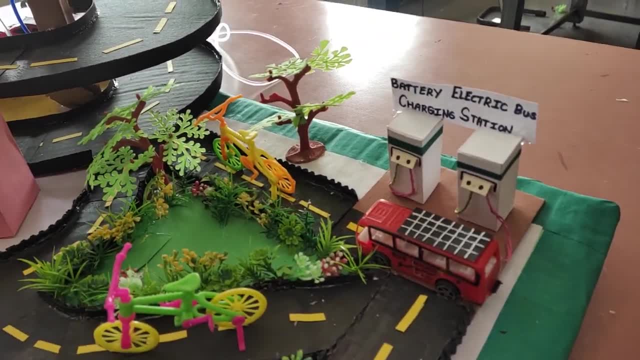 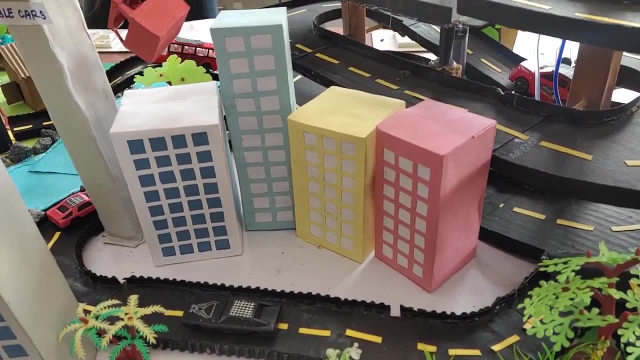 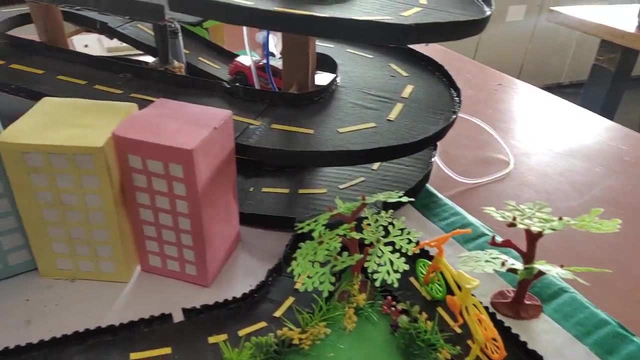 via electric charging station system. this energy for these buses is stored in a battery to be supplied to the electric motor. three types of batteries are commonly used in battery electric buses. they are: lithium, iron, phosphate, lithium, titanate and mike and nickel, cobalt, manganese, lithium, iron. using these electric buses, one can travel around the 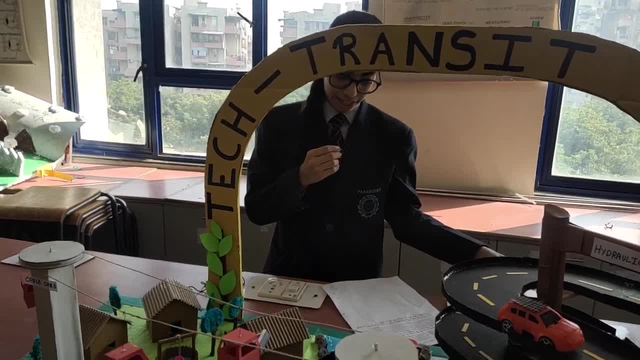 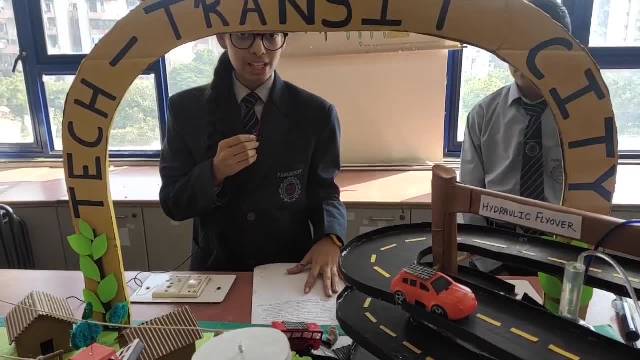 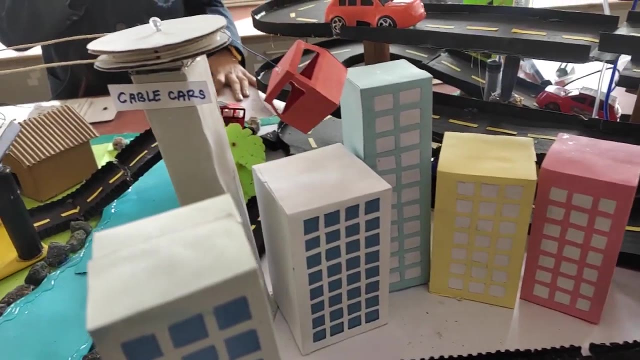 city. in the city, most of the vehicles run on solar energy. and apart from using solar vehicles, people also use electric bicycles. electric bicycles runs on electricity. they use a motor to assist the movement of the paddles. the battery powers the motor. power flows from the battery to the motor.